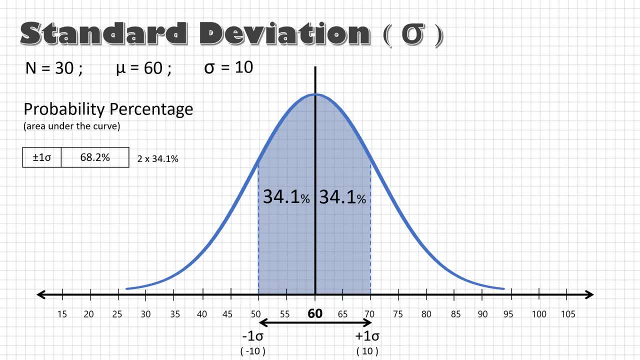 total parts produced with this process are going to be within 50 and 70. That's right area under the curve equals to probability percentage. In the same way, with plus minus 2 sigma, the total area covered for the parts between 40 and 80 will be 95.5 percent. 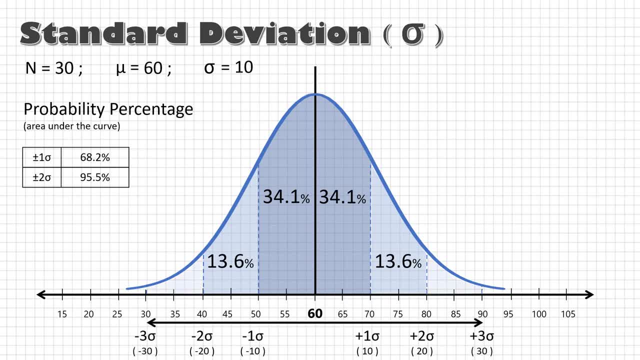 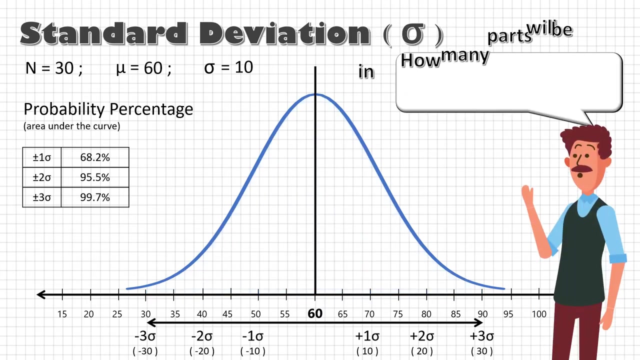 And for plus minus 3 sigma it will become 99.7 percent. That means in any normal process there is a probability that 99.7 percent of the parts will lie within plus minus 3 sigma range. Similarly, if I want to know what is the probability of making parts between 64 and 68,, 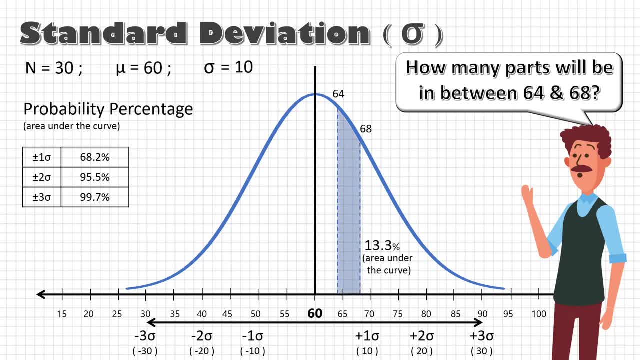 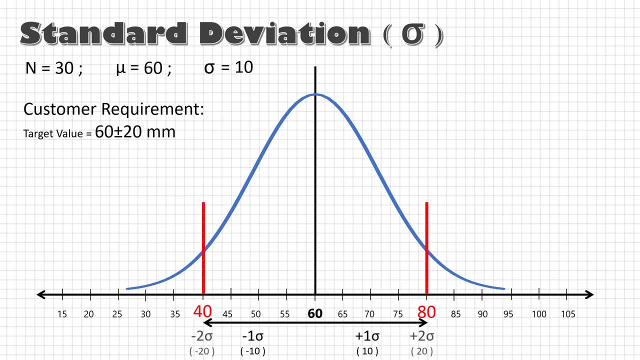 it will be equal to the area under the curve. This is amazing. With the help of just 30 parts, we have predicted the behavior of the process. So if the customer needs part between 40 and 80,, this process can be called as 2 sigma process. 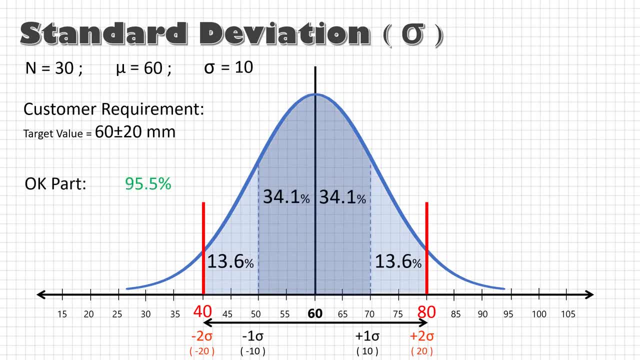 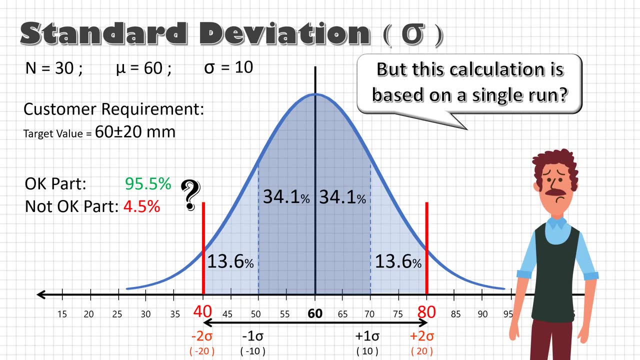 And we may estimate that 95.5 percent parts will be okay and only 4.5 percent are going to be rejected. Actually, there is a catch: This process curve is based on 30 parts that were made in a single run. However, 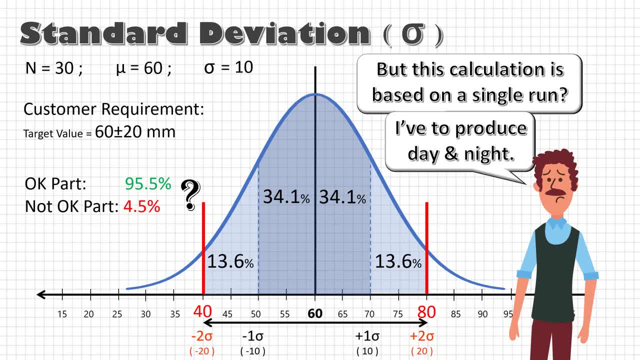 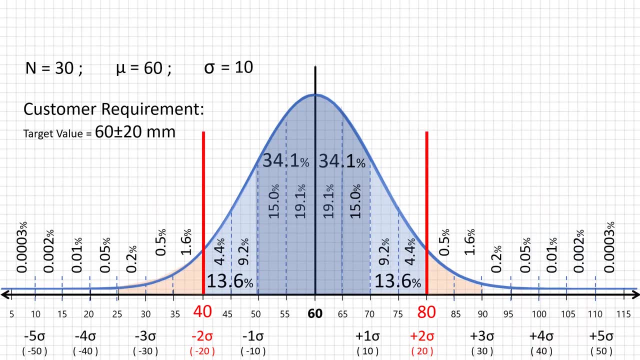 if I were to produce a million parts. variation may occur due to some common causes like operator change, material change, equipment maintenance condition. So there are chances that more parts will fall out of the range To account for this common cause variation, a concept of 1.5 sigma. 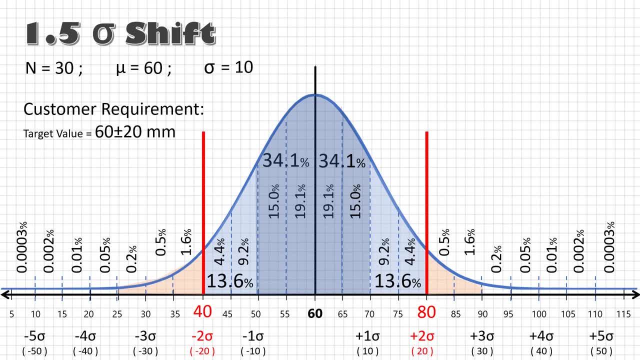 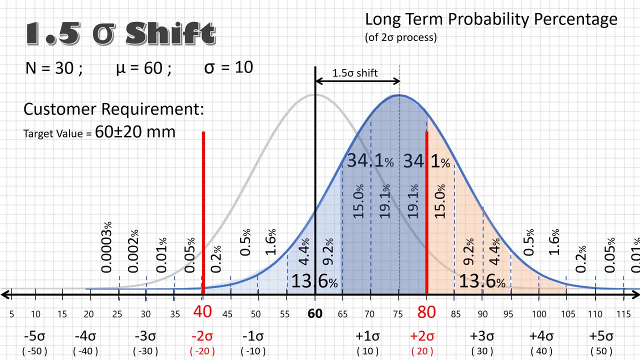 shift is introduced. That means in this 2 sigma process where the probability percentage is 95.5 percent, I have to move the process location by 1.5 sigma to make adjustments for the common cause variation, And by doing so my probability percentage between 40 and 80 drops to 69 percent and the defect ratio